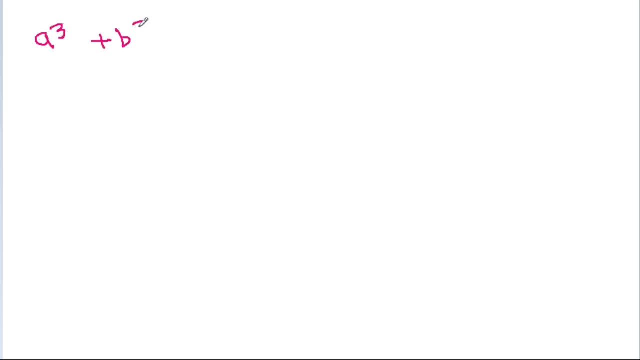 have given that aq plus bq is equal to 7 and aq plus bq is equal to a plus b, into a square plus b square. minus a b, that is equal to 7 and a plus b is x times a square plus b square is x square. 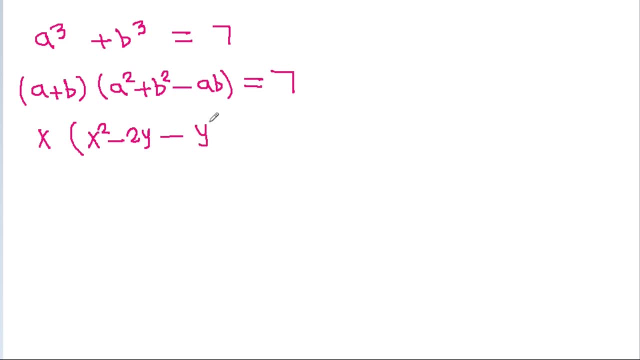 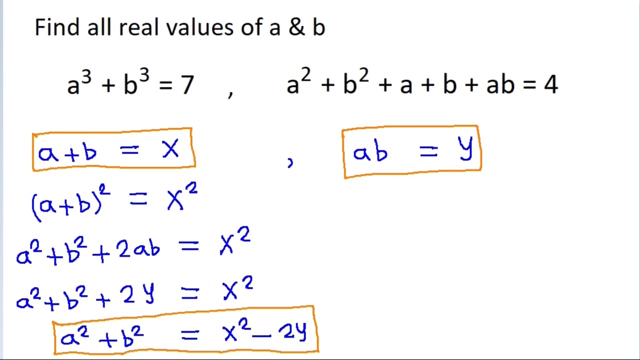 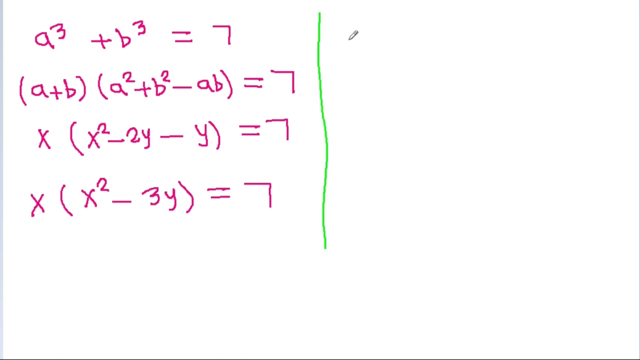 minus 2y minus a b is y, that is 7. or we get x times x. square minus 3y is equal to 7 and we have also given that a square plus b square plus a plus b plus a b is equal to 4. we have given that a. 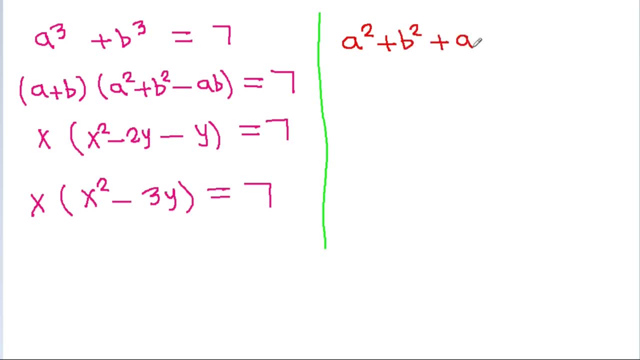 square plus b, square minus a plus b plus a b is equal to 4 and a square plus b square is equal to x. square minus 2y and a plus b is x and a- b is y. that is equal to 4 and we get x square plus x minus y is equal to 4, or we 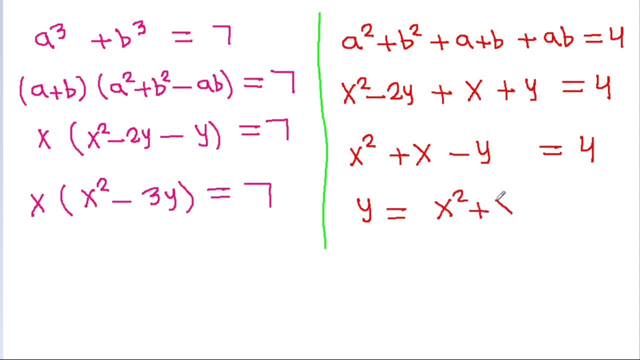 get: y is equal to x square plus x minus 4.. And now if we take this as equation 1 and this as equation 2, and now if we put the value of y in equation 1, putting the value of y in equation 1, then we get x times x square. 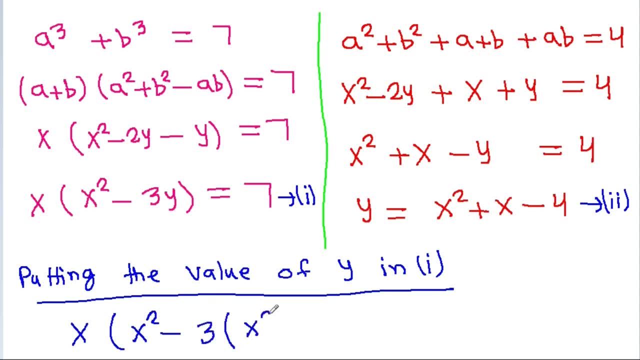 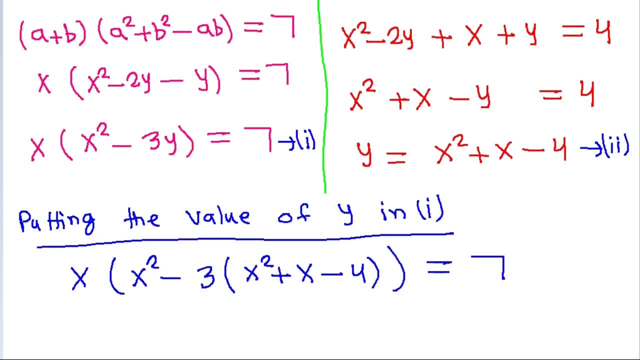 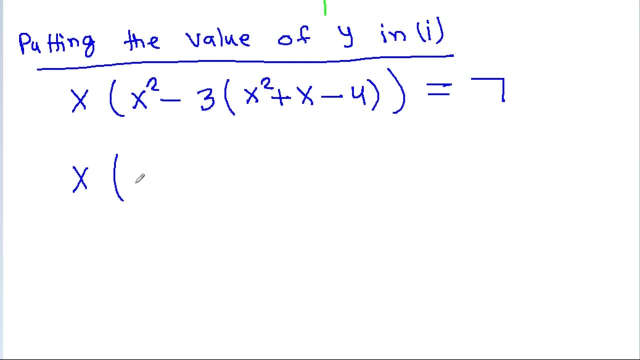 minus 3 times and y is equal to x square plus x minus 4, that is equal to 7.. And we get x times x square minus 3. x square will be minus 2. x square minus 3. x plus 12 is equal. 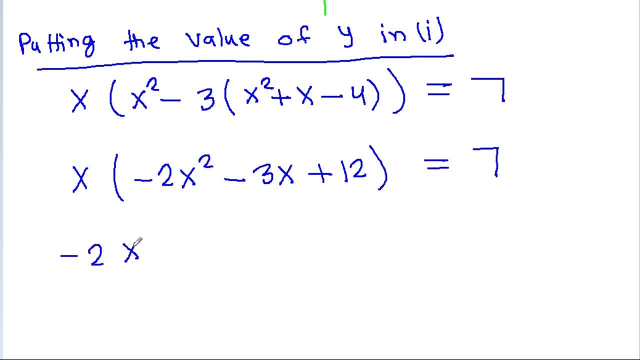 to 7. or we get minus 2 x cube minus 3 x square plus 12 x is equal to 7, or we get 2 x cube plus x square minus 3 x square minus 12 x plus 7 is equal to 0.. 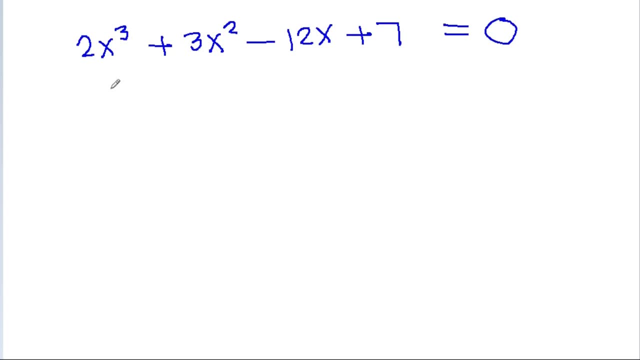 And now, if we put x is equal to 1, then we get 2 plus 3 minus 12 plus 7, that is 0.. So x minus 1 will be a factor. and now for second factor: for 2 x cube we need 2 x square. 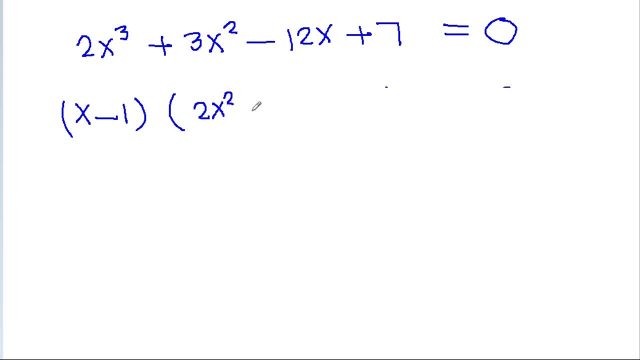 and now for 3 x square we need plus 5 x and for minus 12 x we need minus 7. that is equal to 0 a and we get x minus 1 times. it is 2 x square plus 7x minus 2 x minus 7 is equal. 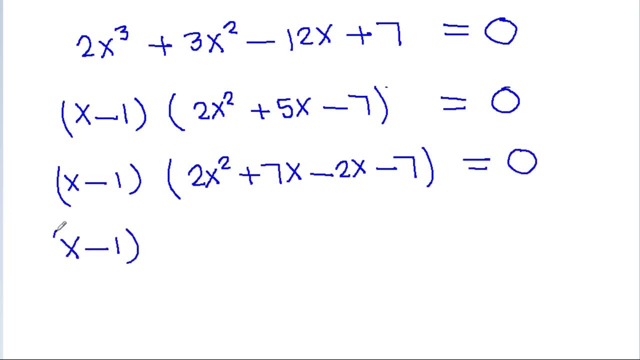 to 0. And we get x minus 1 times 1 times. if we take x common, then we get 2x plus 7, and here, if we take minus common, then we get 2x plus 7 is equal to 0. or we get x minus 1 into x minus 1 into 2x plus 7 is equal. 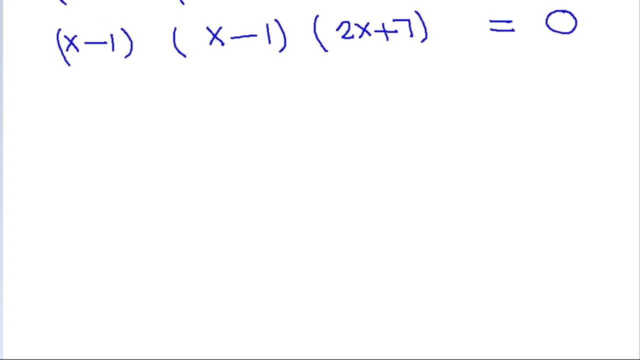 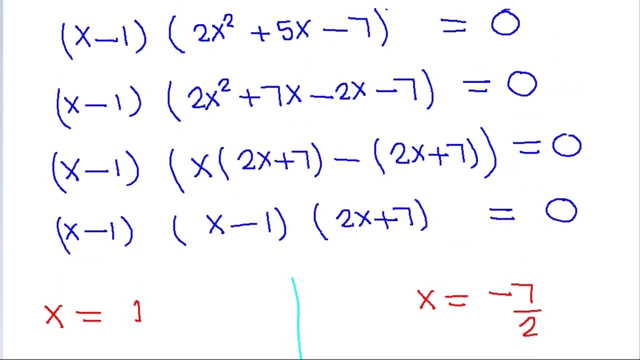 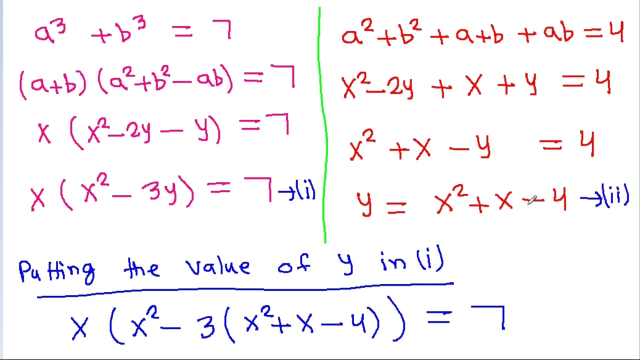 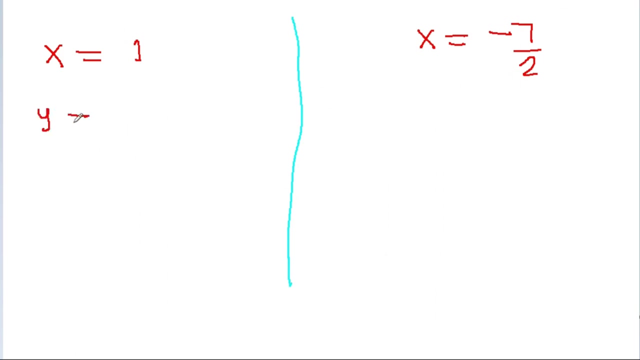 to 0, and now we get: x is equal to 1 and x is equal to minus 7 by 2, and we have: y is equal to x square plus x minus 4.. Ok, We have: y is equal to x square plus x minus 4.. 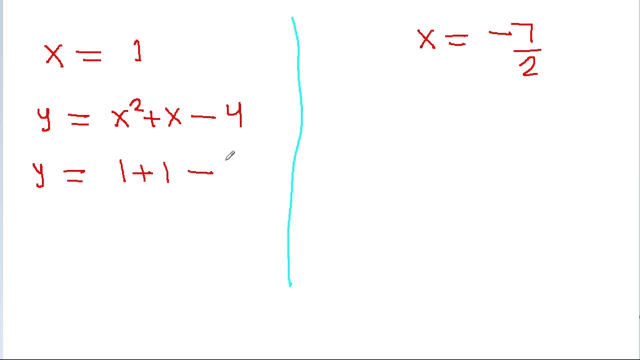 So we get y is equal to 1 plus 1 minus 4, or y is equal to 2 minus 4 is minus 2, and here also we have y is equal to x square plus x minus 4 and we get y is equal to minus 7 by. 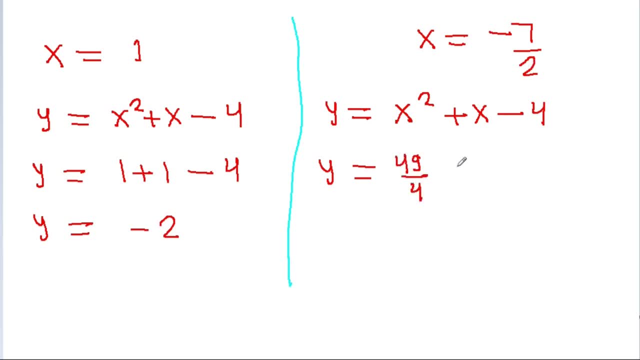 2 square is 49 by 4. And minus 7 by 2 minus 4. And it is y is equal to 4, will be ncm and 49 minus 14 minus 16 and it is 19 by 4.. 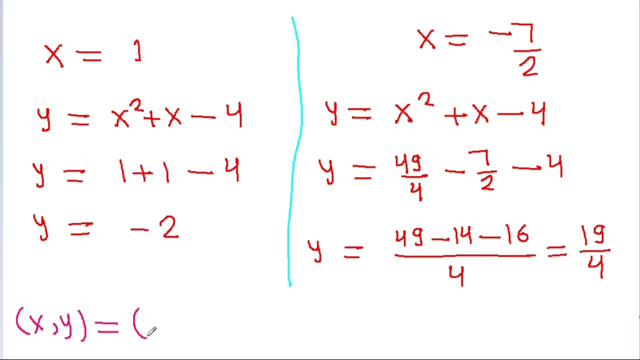 So here we get: x and y is equal to 1 and minus 2, and here we get: x and y is equal to minus 7 by 2.. So this, this is n and we get, we get two plus 2. And 19 by 4.. 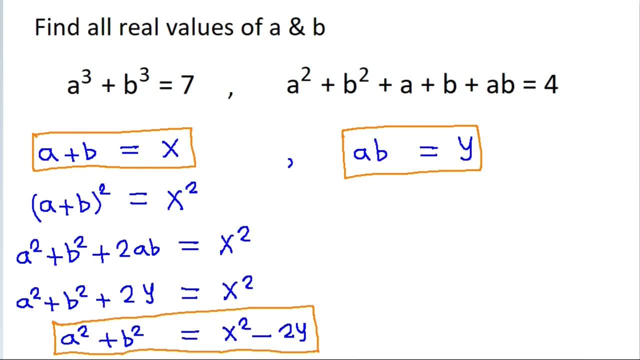 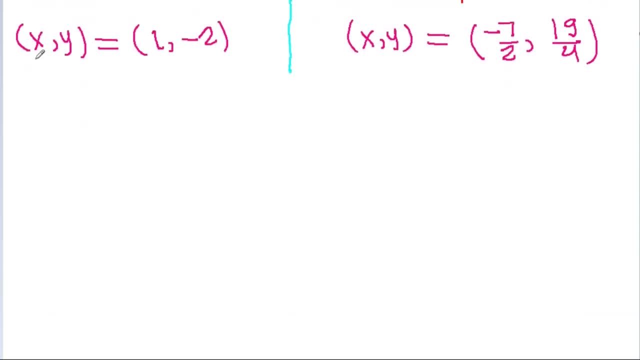 And we have: x is equal to a plus b and y is equal to a into b. We have x is equal to a plus b. So we get a plus b is equal to 1.. And y is a into b. we get a into b is equal to minus 2. and here we get a plus b is equal to minus 7 by 2, and 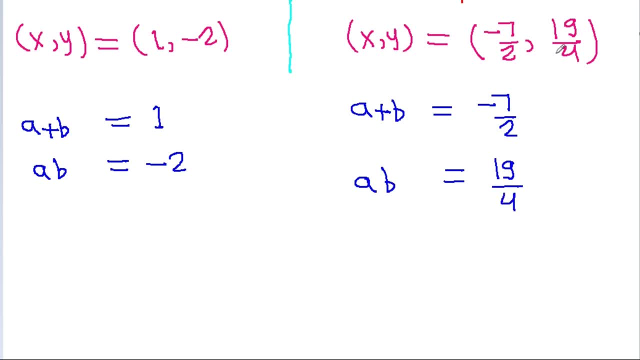 a into b is equal to 19 by 4. and now we have a plus b and a into b. so the quadratic equation having root a and b will be: t square minus sum of root, that is 1 times t plus product of root, that is minus 2, is equal to 0. and here the quadratic equation having root a 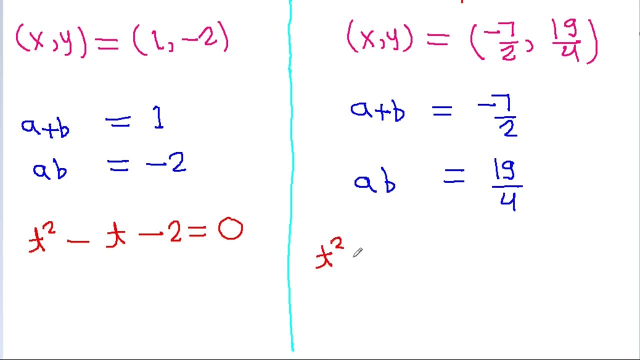 and b will be t square minus sum of root, that is, minus 7 by 2. so we get plus 7 by 2 times t, and product of root, that is 19 by 4, is equal to 0. and now here we get t square minus 2t plus.